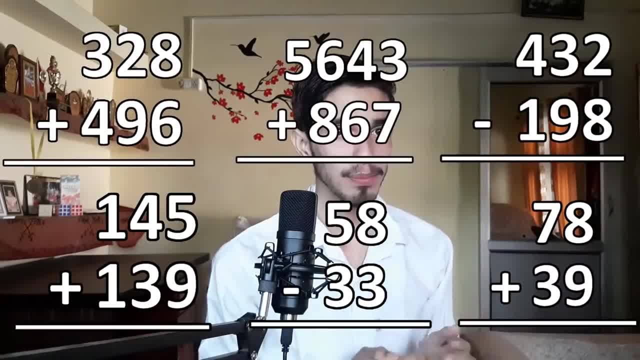 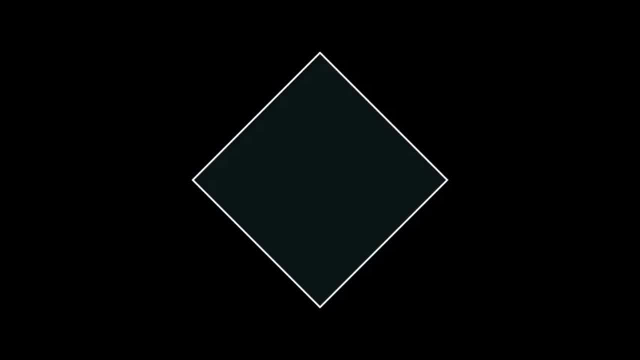 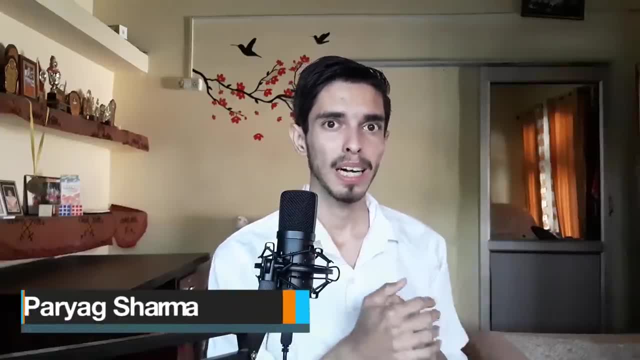 Till the end of this video, you will be able to add and subtract numbers in your head faster than you could ever imagine. So let's begin. Hello Geniuses, Welcome to the second part of MathoGenius Mental Math Series. In this, 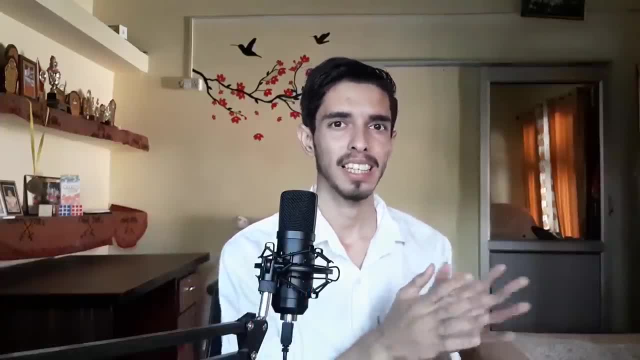 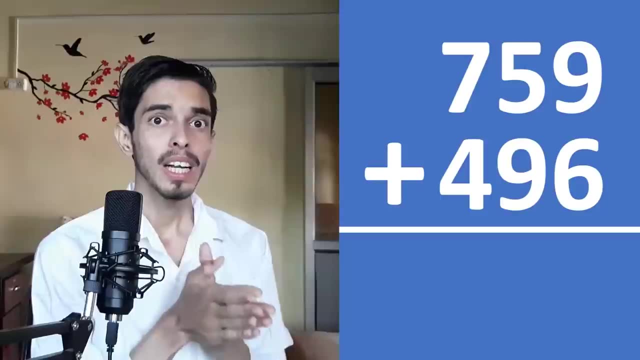 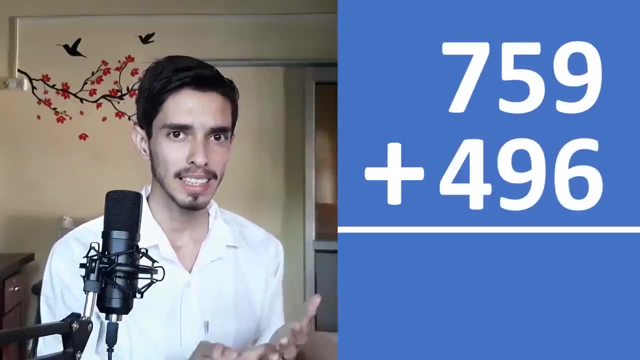 video we will learn how to add and subtract numbers lightning fast. So I have a question for you: Add 759 and 496 in your head right now and note that time Okay. so this is how most people would do it. They will imagine 759 and 496, then they will add 9 and 6 and 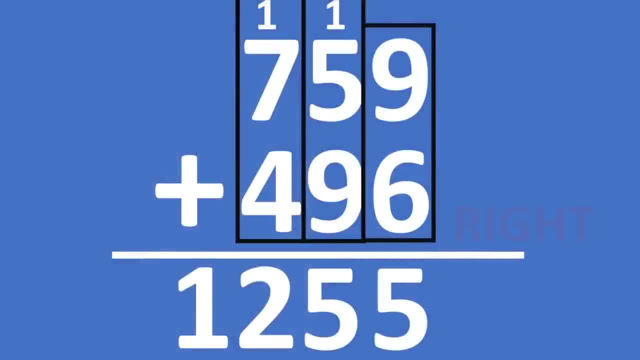 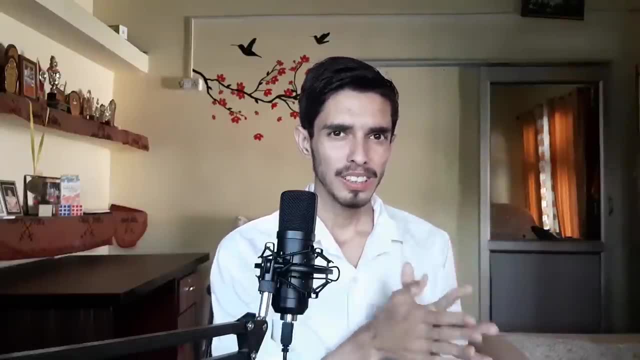 then they will take the carry and so on. Basically, they will go from right to left, And this is basically what we learn in school. But what if I tell you this is the worst way to do it, if you are doing it mentally On paper? 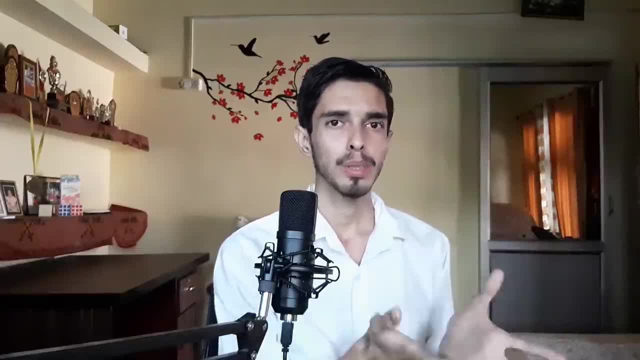 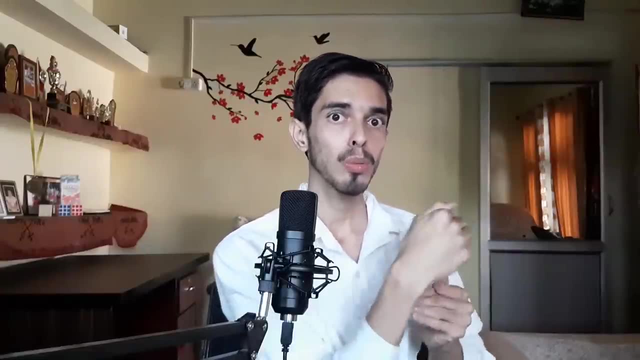 it is fine, but for mental maths this is the worst way, Because see how do we read numbers From left to right, And in here we are going from right to left. So this is the exact opposite that our brain is trained to do. So this is not the right way of doing. 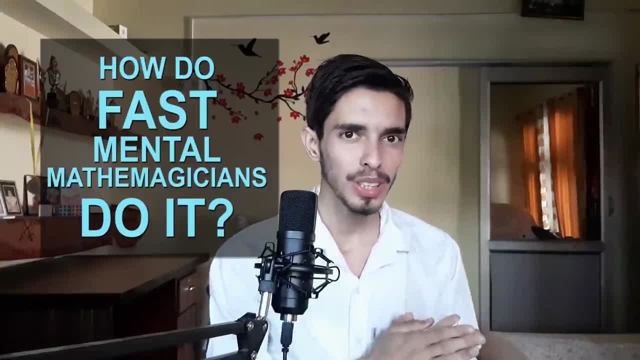 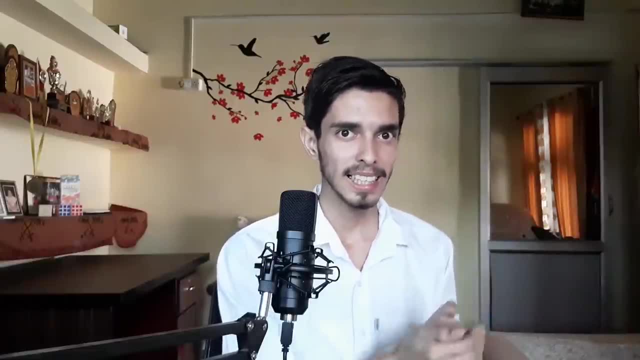 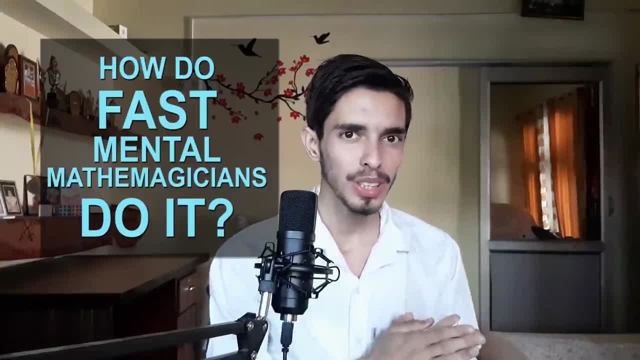 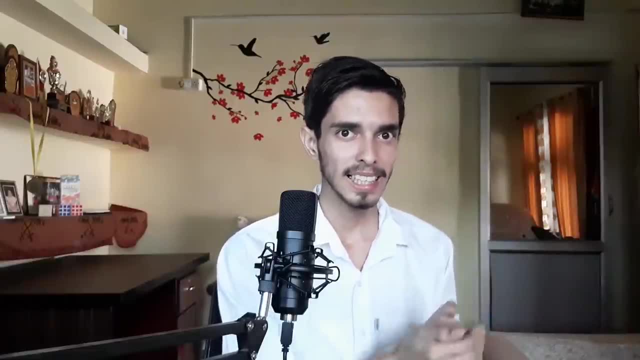 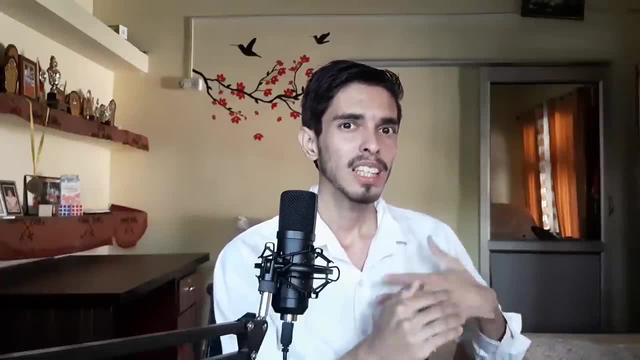 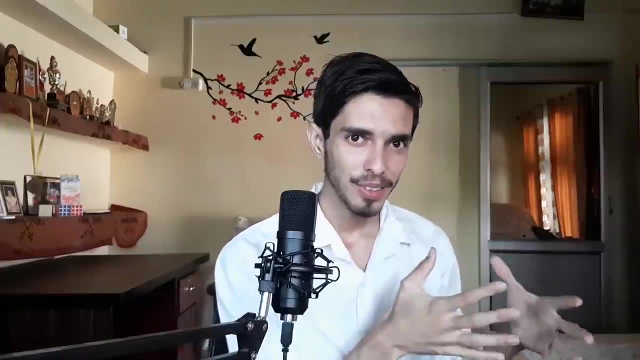 if you have a question, you can just say it. For example, if you have a question, you compute the last digit first and we can't just say it. but in this method we can just say it and give a faster than calculator illusion. So this is how to add 759 and 496, mentally, Instead of 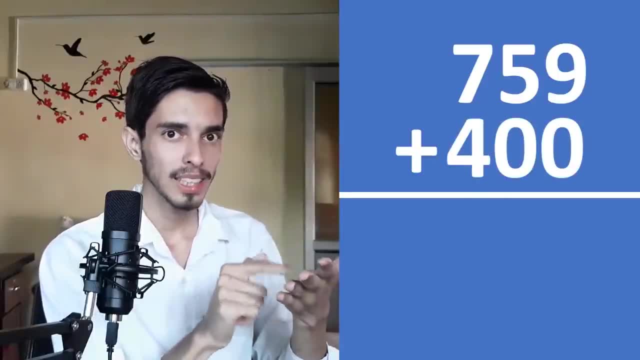 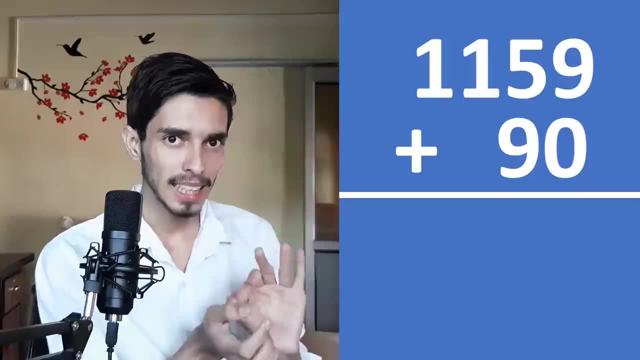 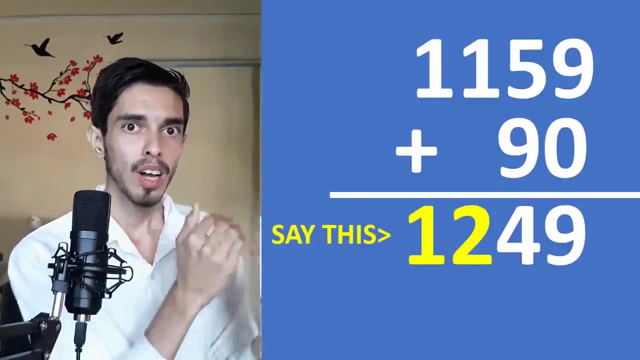 adding 496, add 400 first. So 759 plus 400 is 1159.. Now add 90.. So 1159 plus 90 is 1249.. Now in here, 12 is our final answer, So we can just say it 12.. Now people will think that we have computed the. 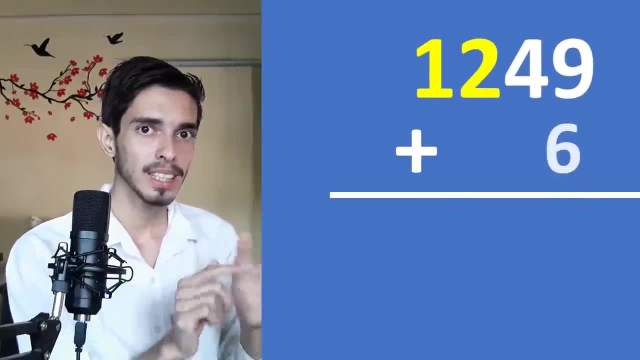 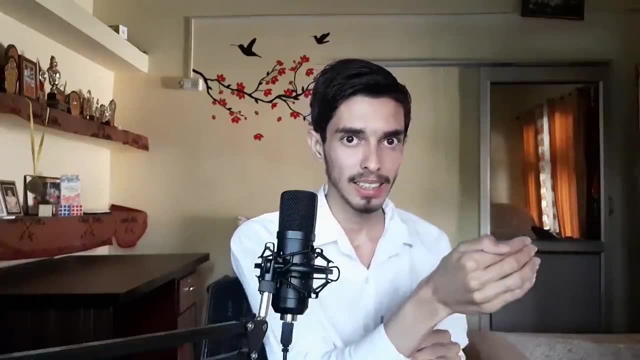 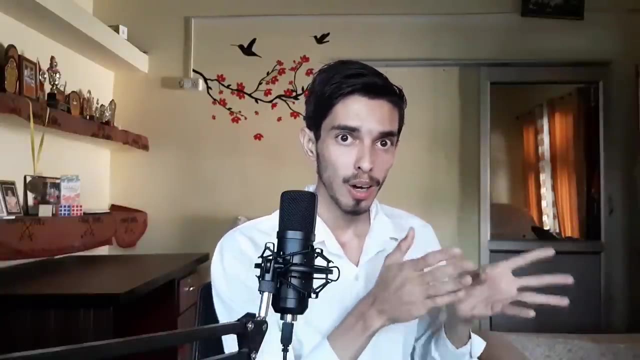 whole answer, but we need 49 plus 6, which is 55.. So 1255 is our final answer. Now, before getting the final answer, we have said 12.. So people would think that we have calculated faster than a person with a calculator. So this is how mental mathematician give the illusion that they are. 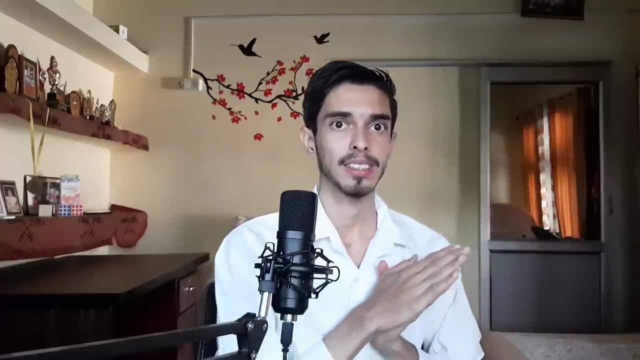 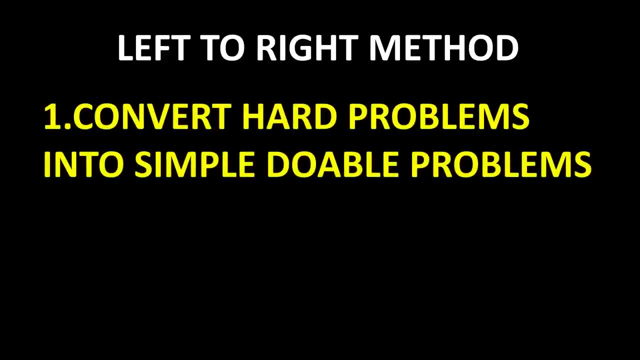 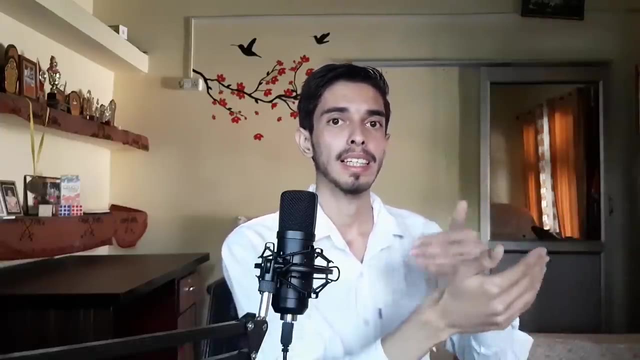 faster than a calculator while calculating their answer. Now, the main principle of this left to right method is that we basically convert hard problems, which your mind can't solve, to simpler, doable problems, and as we compute our answer, the problem becomes easier and easier, and this is why this method is used for mental addition subtraction, also for 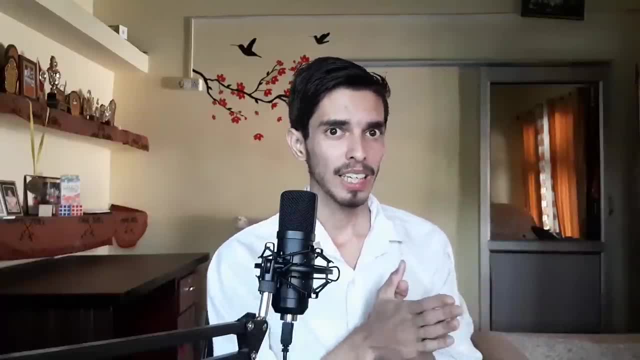 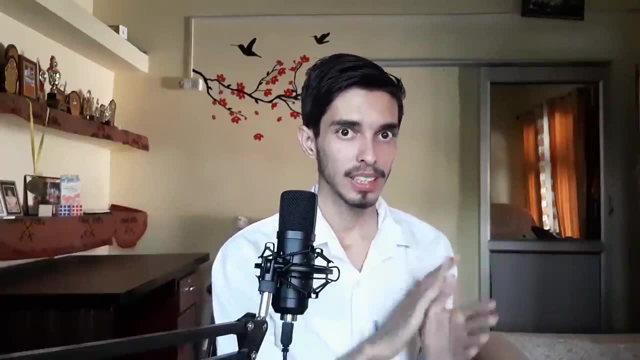 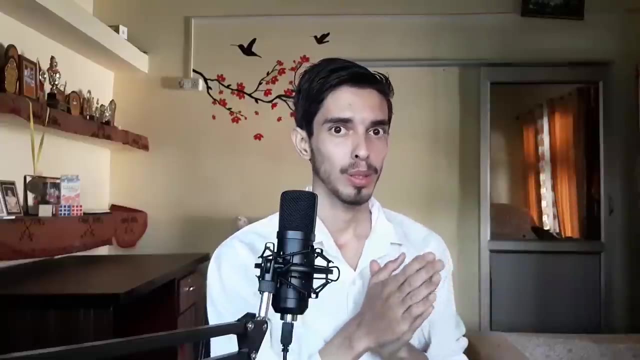 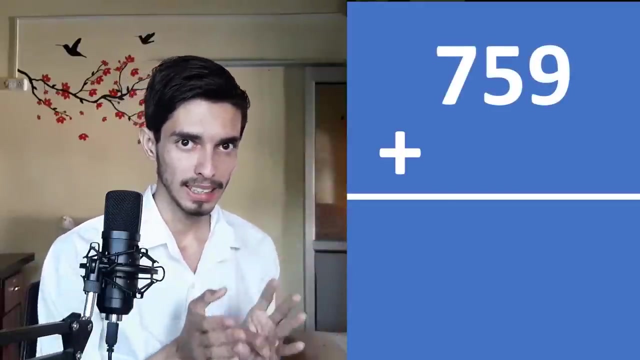 multiplication and division. So always remember that every fast mental mathematician always go from left to right. They never go from right to left. So in left to right method we need to convert hard problems into simpler doable problems. So see that same problem, 759 plus 496, can be done in a more simpler way: See 759 plus 496.. Instead of adding 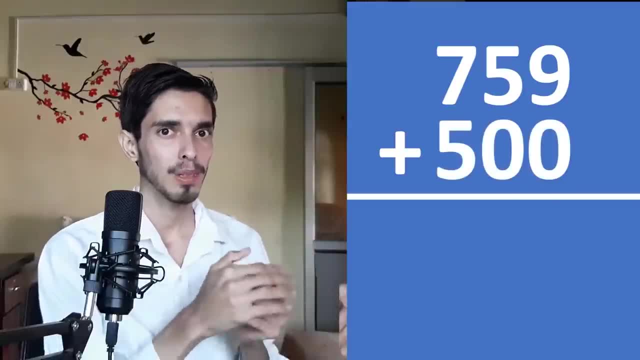 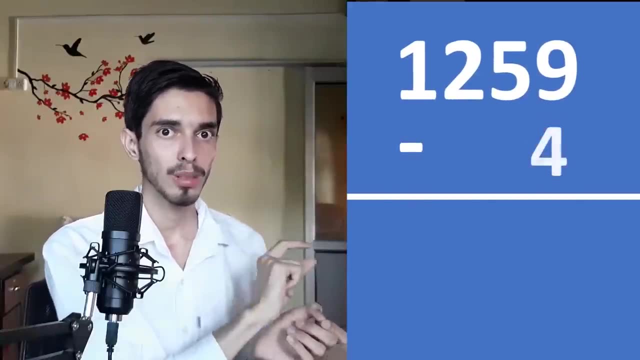 496, let's add 500.. So 759 plus 500, which is 1259.. Now in here we have added 4 more, So let's subtract 4.. So 1259 minus 4 is 1255, which is 1259.. Now in here we have added 4 more, So let's subtract 4.. So. 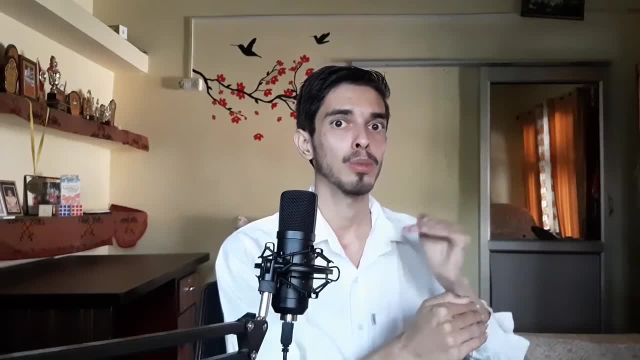 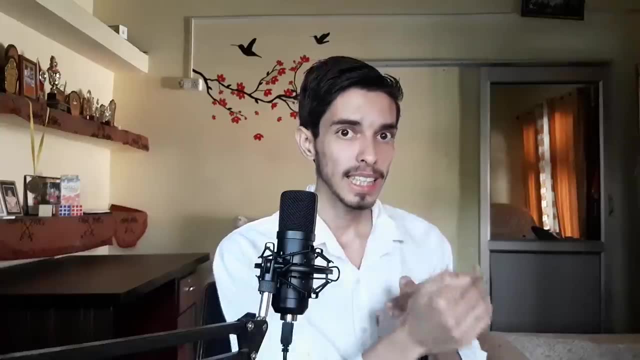 this is our answer. So this is how fast we can do it if we are more creative. So rule number two of this left to right method is that always be creative. The more creative you are, the more you will give the illusion that you are faster than a calculator, Because see, in here we have just 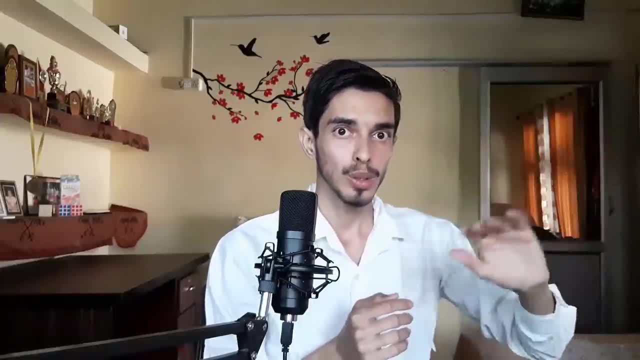 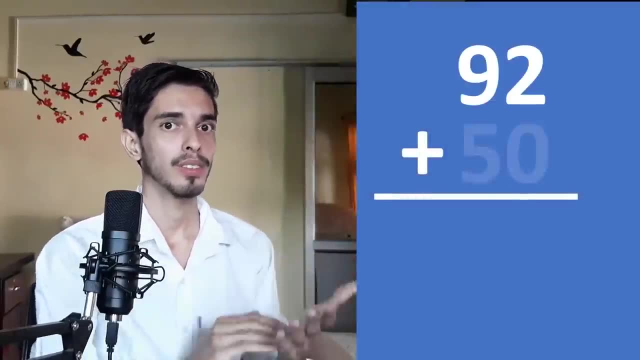 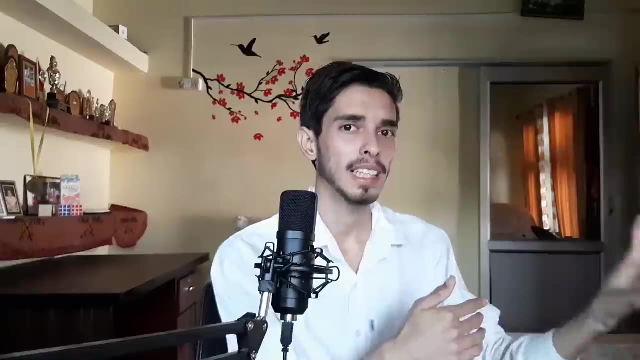 computed 12 in the first second, So we can just say it. So in here we are faster than a person with a calculator. Now try 92 plus 53. So 92 plus 50, which is 142.. Plus 3 is 145.. Now you can say 140 before you have calculated your final answer. Now try this one. 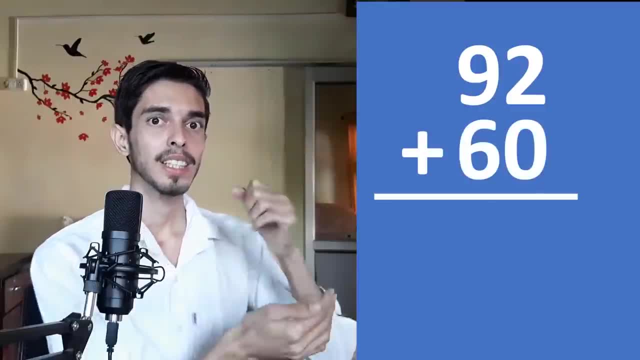 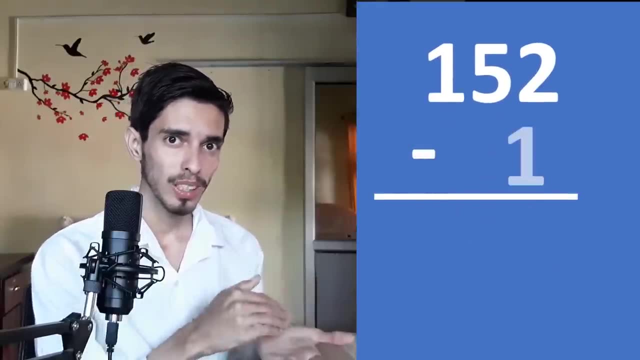 92 plus 59. Now, if you added 60 first, then you are on the right track. So 92 plus 60 is 152.. Now we have added one more, So 151 is our answer. So this is how fast we can do it. Now, as I always say, the. 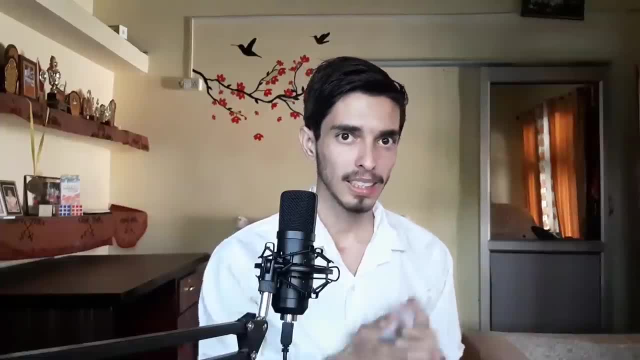 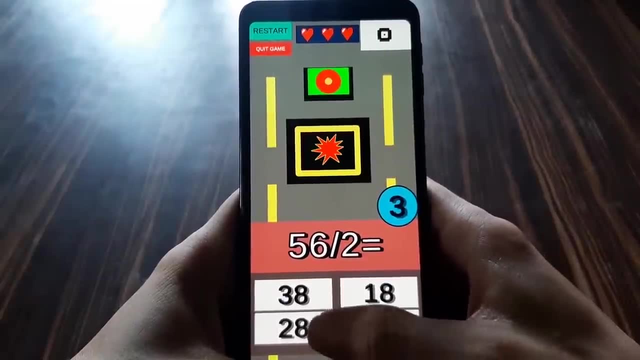 more you will practice, the better you will be in mental maths. So that's why I have created this free game known as Math Blower. In this game, there is a bad blob who is chasing a good blob who wants to eat it And solving mental 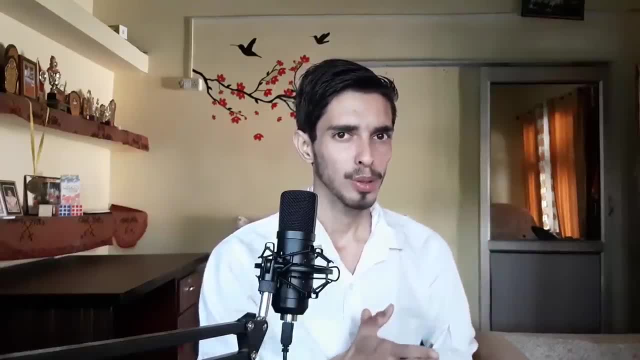 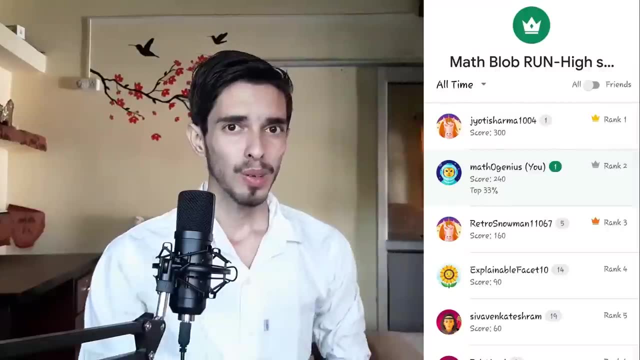 math questions can save your blob, So this game will help you to practice mental maths in a fun way. Download link of this game is in the description of this video. I also added online leaderboards in this game So that you can compare your high score with others and also compete to. 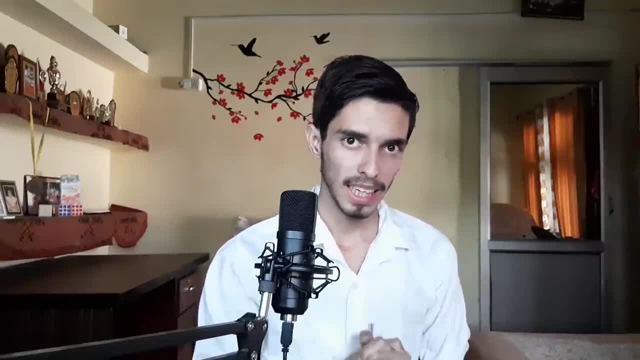 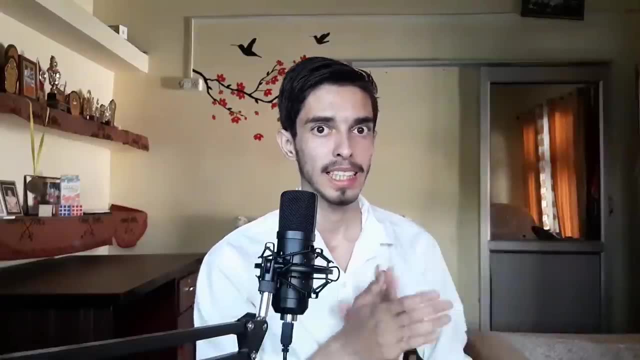 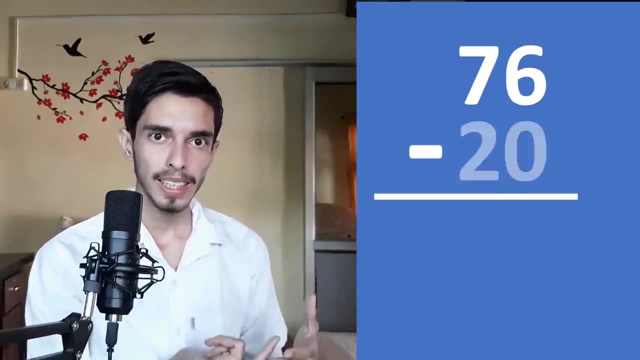 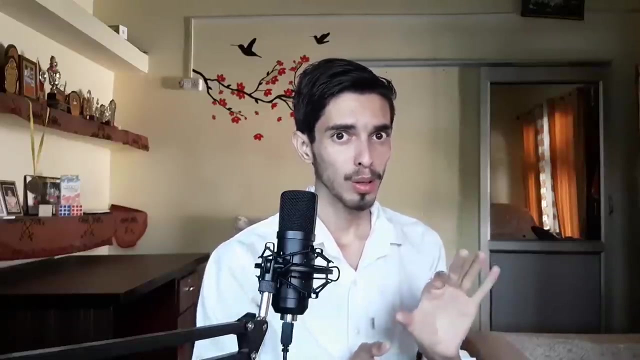 get the number one spot. Now let's see how to do mental subtraction. Same principle here: Always convert hard problems into simpler problems and be creative. So try this one: 76 minus 25.. So now see: 76 minus 20 is 56, minus 5 is 51. That is our answer. Now, if you are creative, you can do this. 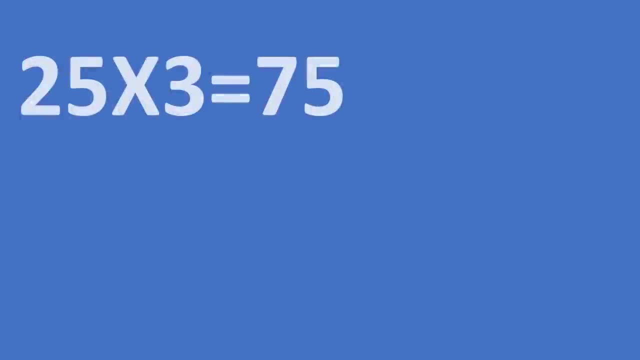 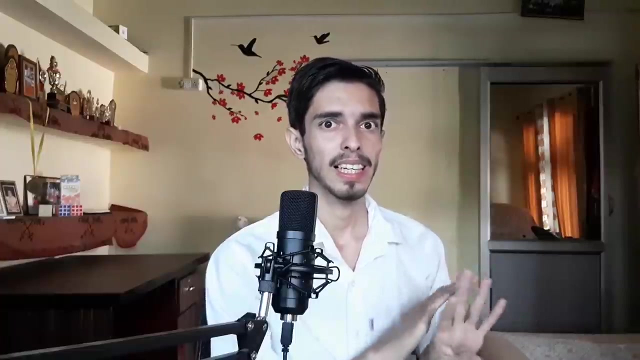 problem without even doing subtraction: See 25: 3s is 75 and 25: 2s is 50. And 76 is 1 greater than 75.. 51 is our answer. Now see, with creativity and practice, you can be faster than any person with. 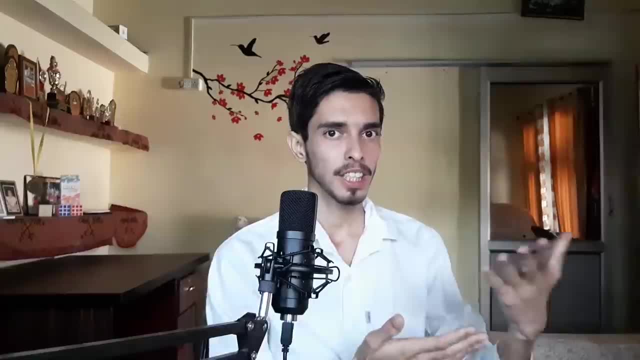 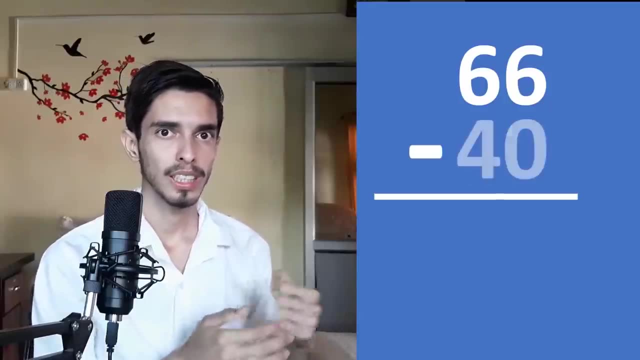 the calculator, Because they would be just chunking the numbers and you will just say the answer. Now, let's try 66 minus 39.. Now, instead of subtracting 39, subtract 40. So 66 minus 40 is 26.. Now we have. 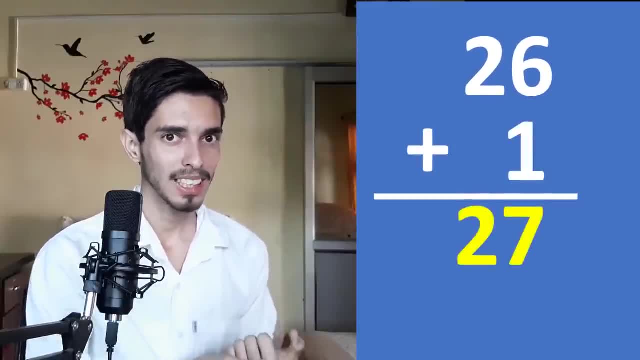 subtracted one more, So add one, So 27 is our answer. So this is how fast you can do it. And also say 20 before computing that 7.. Because this is how fast you can do it, So let's try. 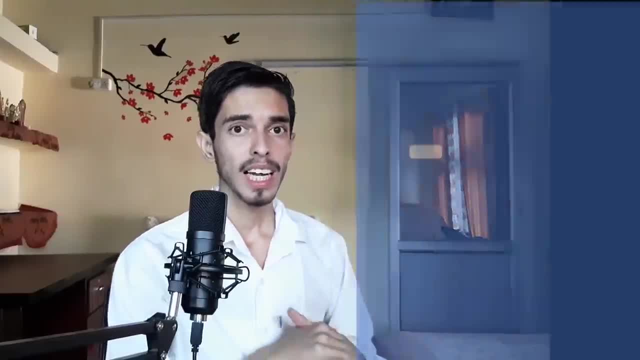 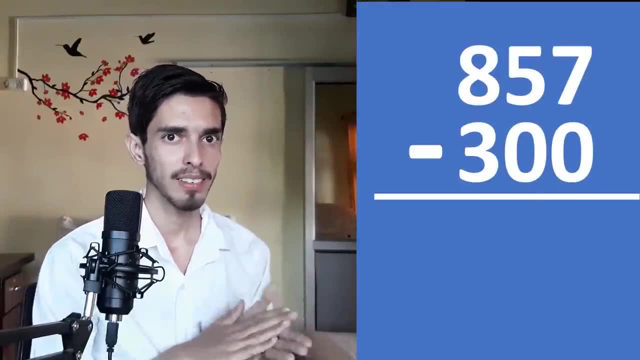 65.. So this will give the illusion that you are faster than a calculator. Now try your mind on 857 minus 298.. Now subtract 300 first, So 857 minus 300, which is 557.. Now add to 557 plus 2 is: 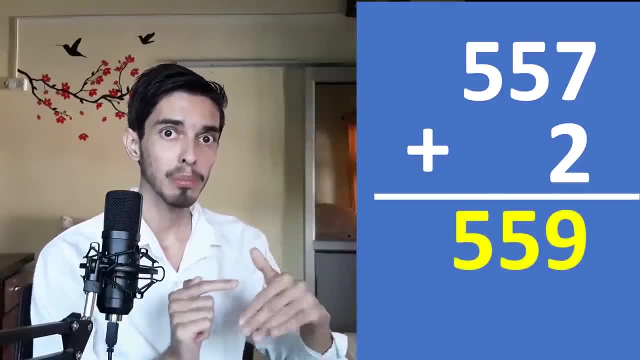 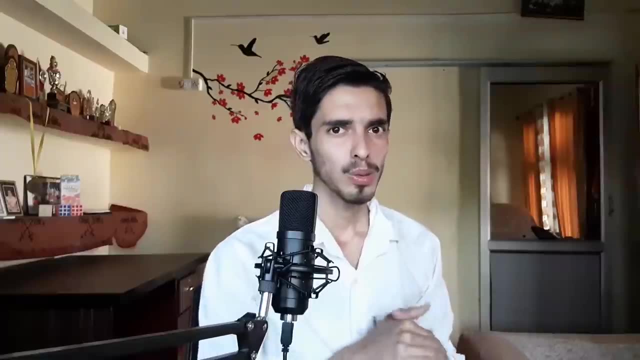 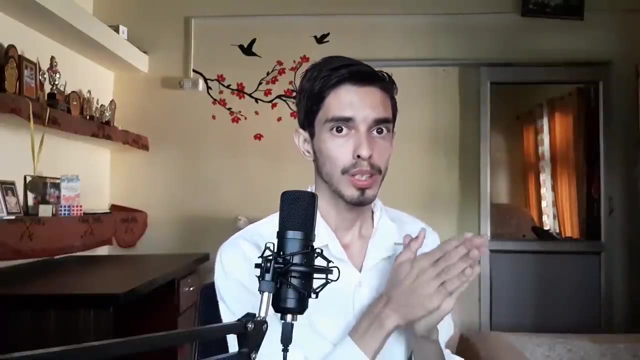 559.. That is our answer, And 550 can be said before computing the last digit, And with that you will be faster than a calculator. Now I have a cool bonus for you, which is known as compliments. This will help you to even be more creative. This method is used to compute how far is the two digit. 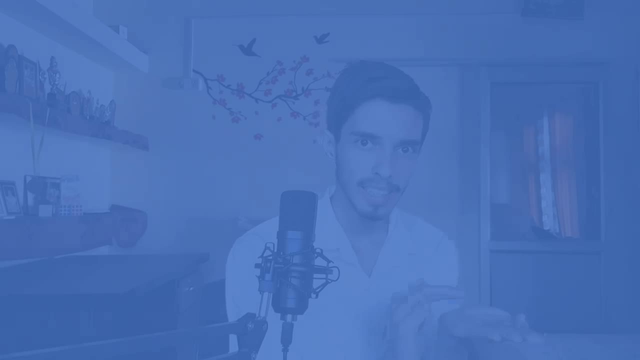 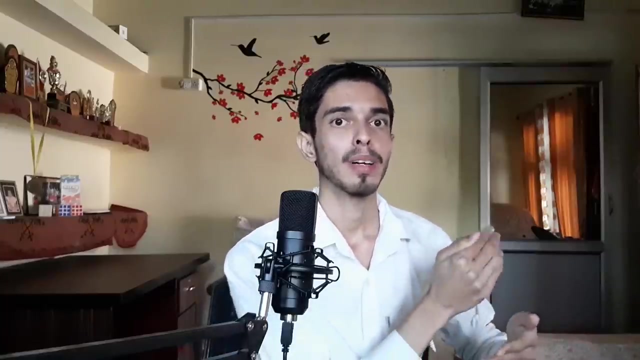 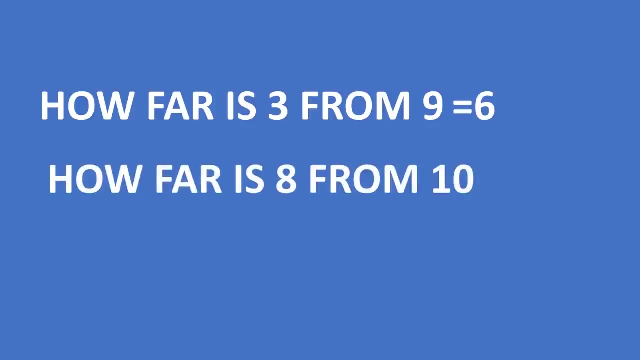 number from 100.. So see how far is 38 from 100, or in other words, how much is 100 minus 38.. So, instead of doing the subtraction, look at this: How far is 3 from 9? 6.. And how far is 8 from 10? 2.. 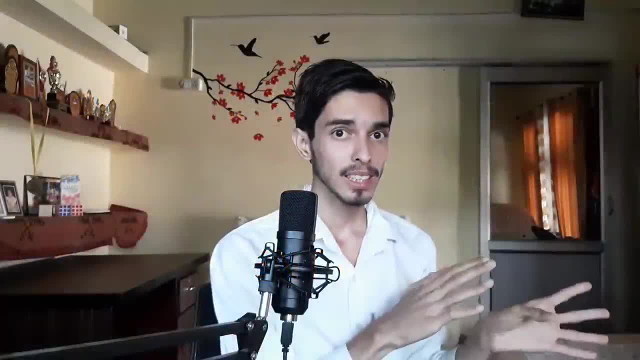 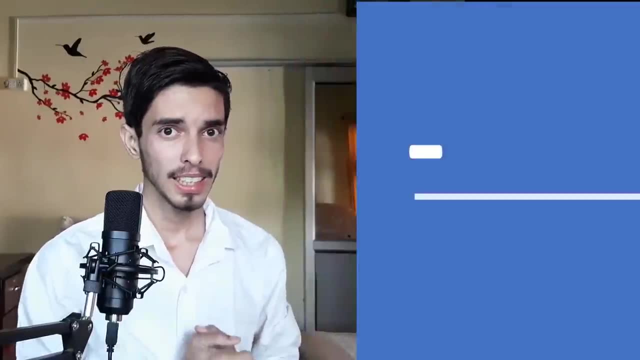 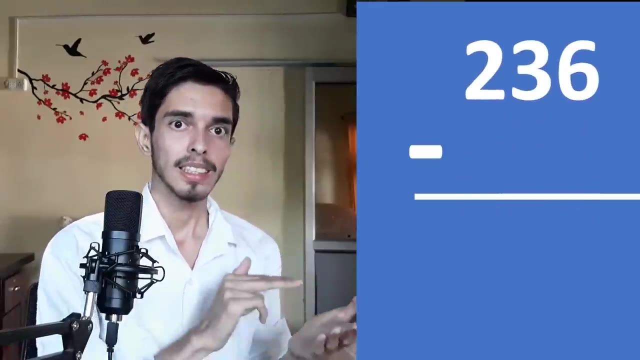 So 62 is the compliment of 38, which is 100 minus 38.. Now let's see how compliments helps us to calculate faster. So see this: 536 minus 378.. Now, if you use the left to right method, you can do this: 536 minus 300, then 70 and then 8.. But this 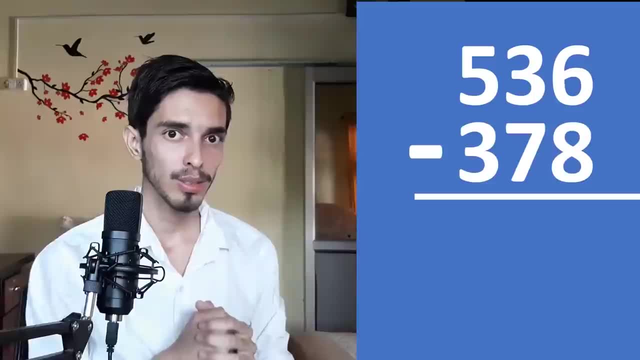 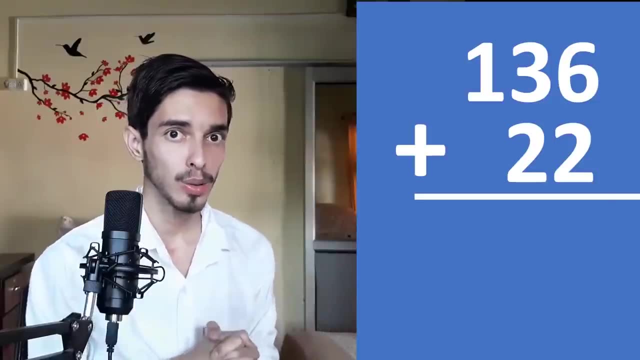 one is a little longer. So what you can do is this: Subtract 400 from 536, which is 136.. Now the compliment of 78 is 22.. So 136 plus 22 is 158.. So this is how compliments help us. 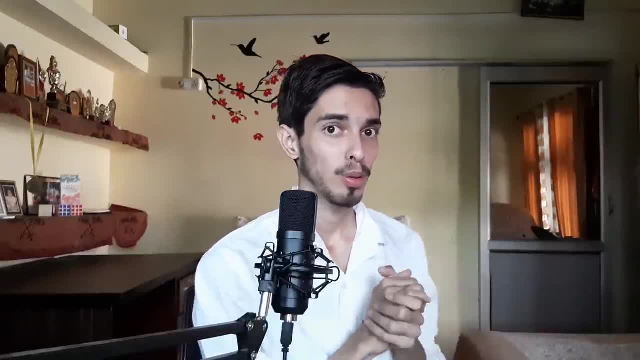 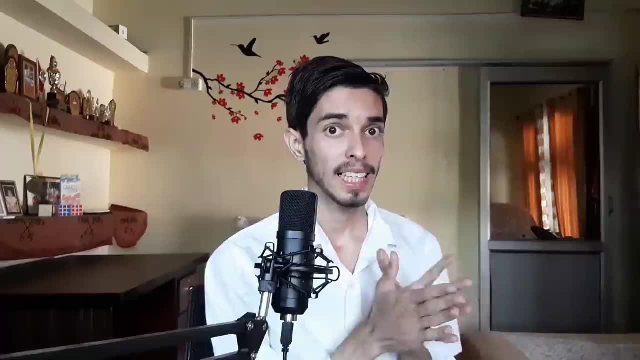 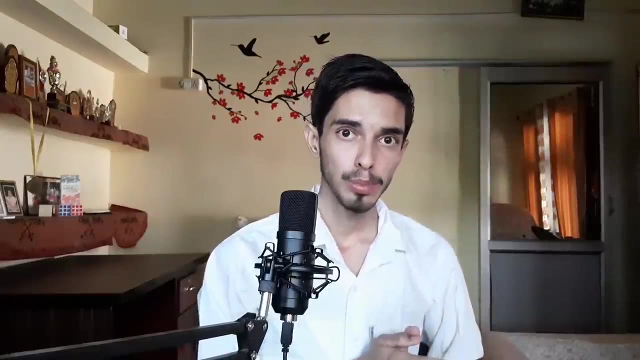 to calculate faster. Now, with this and some practice in math lobe run, You will be able to do any subtraction and addition problem lightning fast. Also, most of the tricks that I taught you are from this book, Secrets to Mental Math, which is a really great book. Buying link of this book.